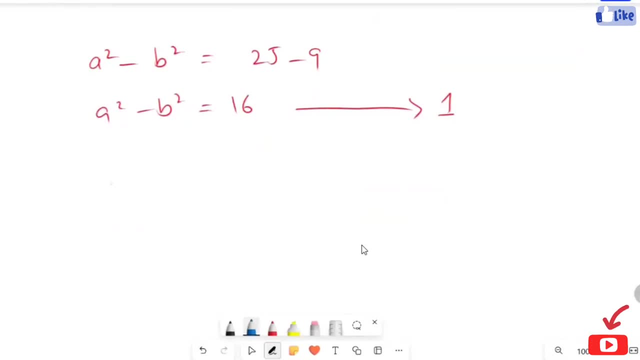 So now I'm going to add up the a- b values, so We will get a square minus b. square is equals to 25 minus 9.. this will dash to, so this is our second expression. now i am going to rewrite our given expression: 5 raised to the power n minus 3. 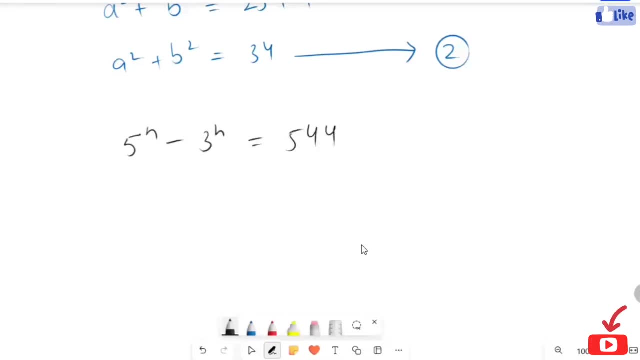 raised to the power n is equal to 5 raised to the power 44. so in replacement of 5 and 3 we already consider a raised to the power n. b raised to the power n is equal to 5 raised to the power 44. 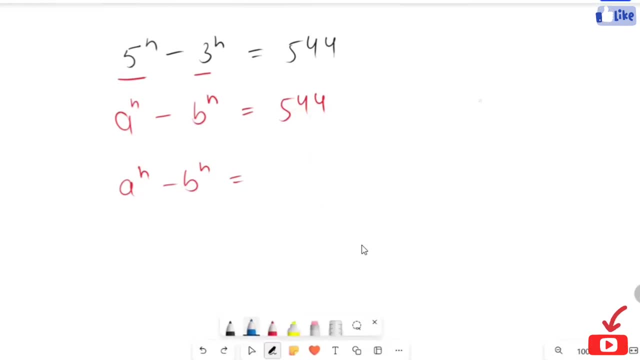 here i am going to find the time factor of 5 raised to the power 44. that will change this. so now this will our take as 2 raised to the power 4, and 2 and 17. so our next expression turn to 2 raised to the power 44. 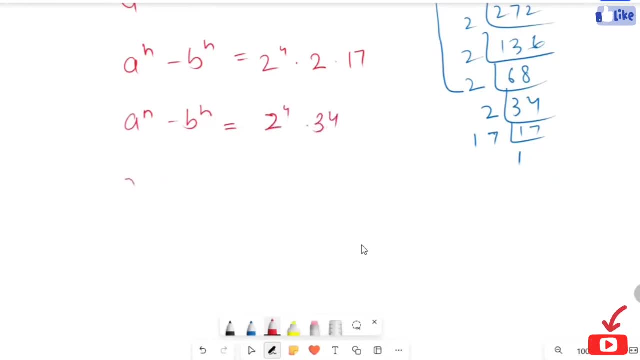 34, 8 raised to the power 1 and 1 raised to the power 0 and 1 raised to the power 0 is equal to 16, 34. now, in replacement of 16, and in replacement of 34, i am going to use our expression 1 and 2. 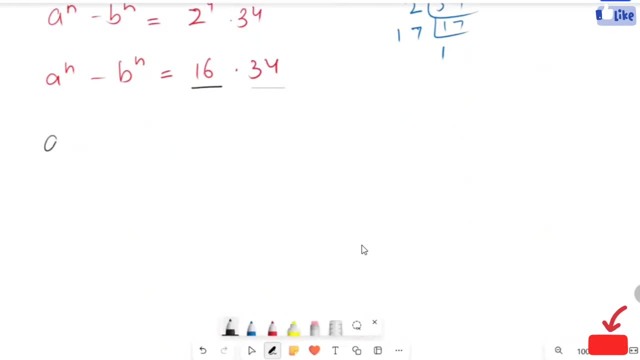 next expression turns to a raised to the power n, and a raised to the power n is equal to a raised to the power n minus b raised to the power 0. a raised to the power 0 will be 2 raised to the power 0. 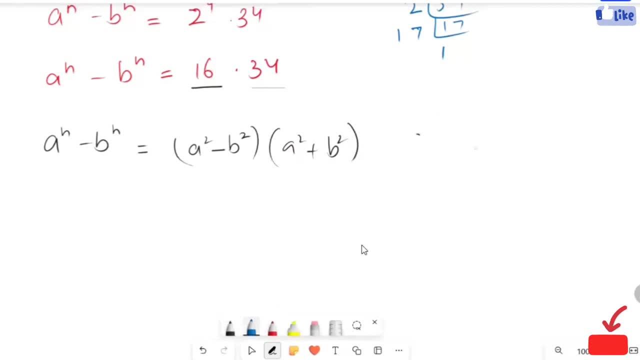 and 3. a raised to the power 1 is equal to a raised to the power 4 and 2 squared, and by adding feathers we will get the expression. so we're so all right. so now i'm going to use the Y stronger now.